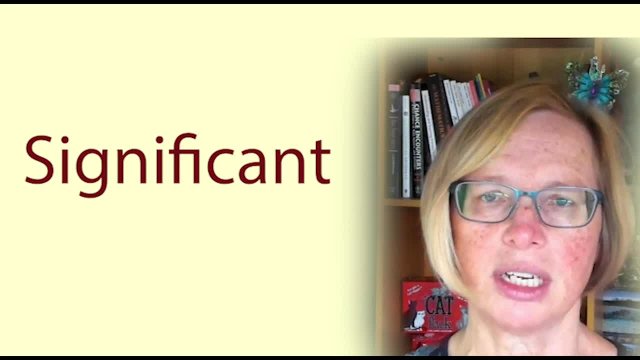 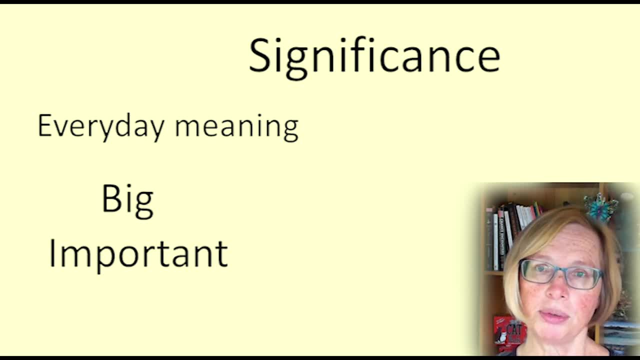 significant is that it has different meanings in everyday language than it does in statistical language. In everyday language, significant can mean big or it can mean important. For example, we could say my earnings are significantly more this year than they were last year. That means that the difference is quite big. So significant in that particular instance means big. 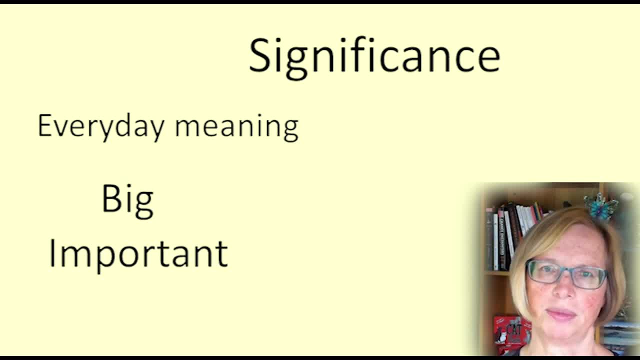 Or we could say that there's been a significant increase in sea temperature. Now that increase is important, but it may be quite small. So those are two everyday meanings of significant. Big and important are the everyday meanings of the word significant, But in statistical analysis the word significant means something quite different. 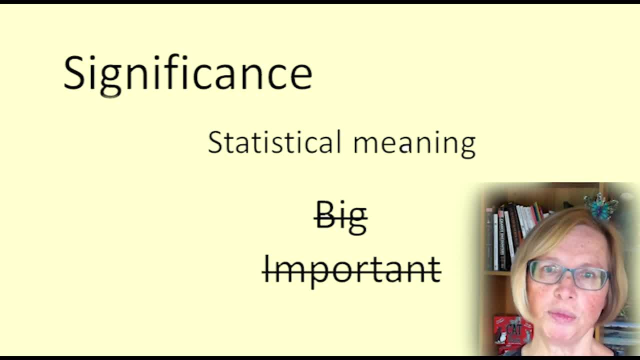 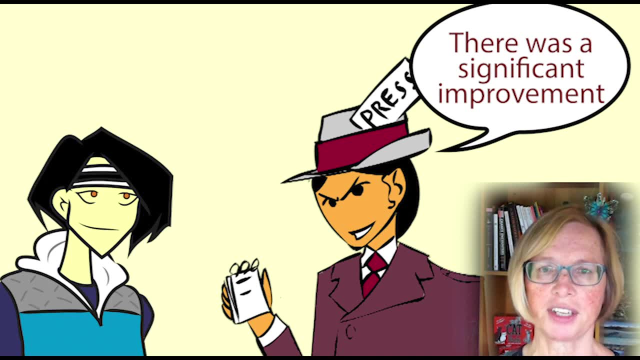 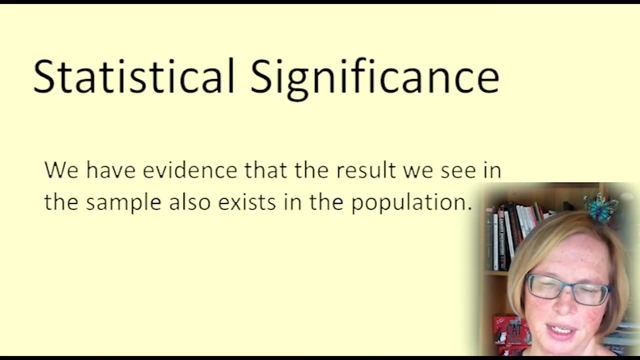 Something can be statistically significant and be small and unimportant. This is a problem with news reports, because when people say that the results are significant, people think that means big and important, But in fact it might not be When a result is statistically significant. 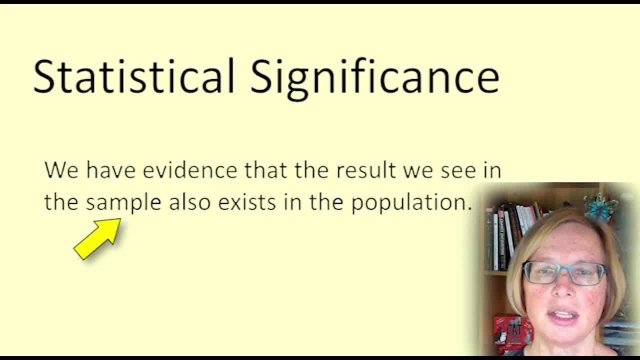 that means that we have evidence from our sample that the effect that's in the sample exists also in the population. Now you need to understand what sample and population are to understand this. so if you don't, it would be good to look at our video on. 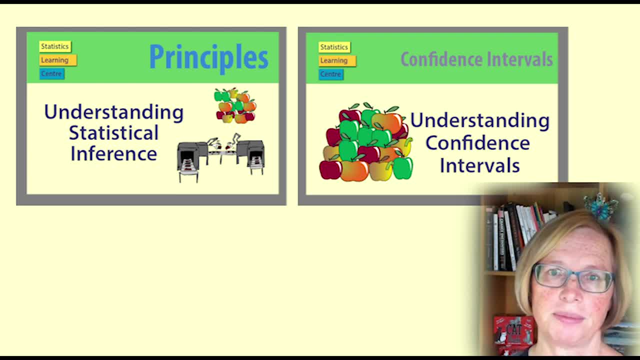 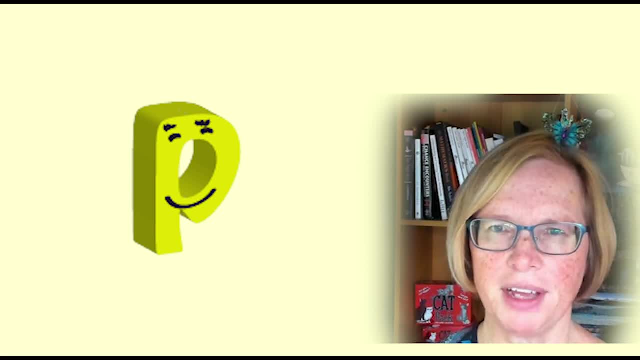 understanding inference or understanding confidence intervals. Generally, we use a p-value to decide if something is statistically significant. We use the p-value to determine if the effect that shows up in the sample indicates that there's an effect in the population, or could it have occurred simply by chance. 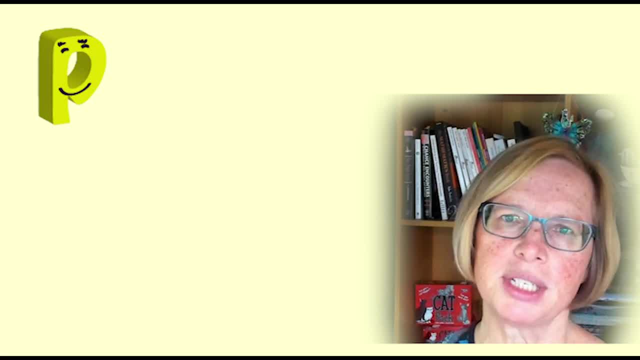 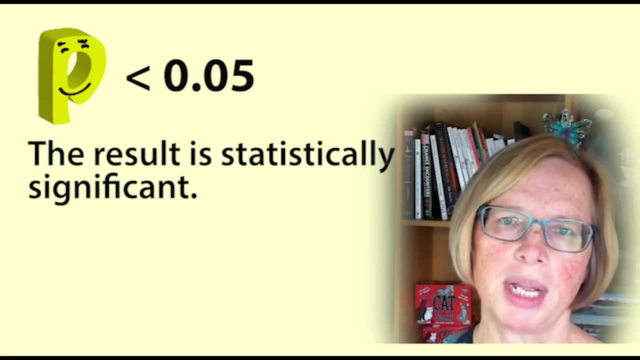 or by sampling error. Generally, when a p-value is less than 0.05, we say that the result is statistically significant. We have evidence that the effect exists in the population. When we reject the null hypothesis, which is that there is no effect, we are saying that there is an effect and that the result is. 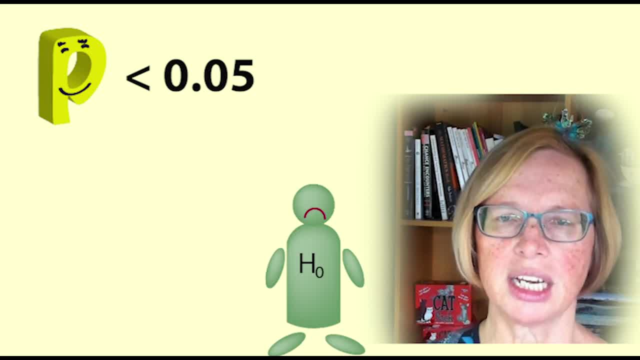 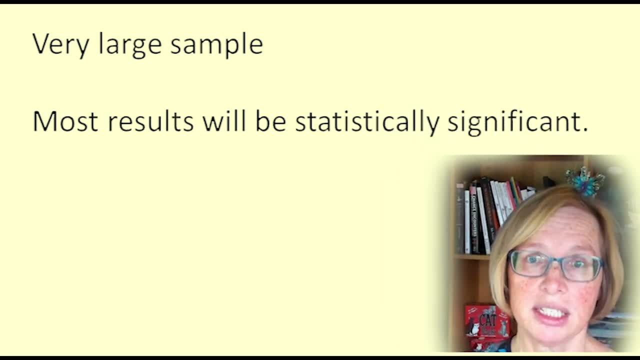 statistically significant. So low p-value: reject the null hypothesis. statistically significant result is 0.05.. If you have a really large sample, then just about anything is statistically significant. You can have a very small effect. but because our sample is so big,